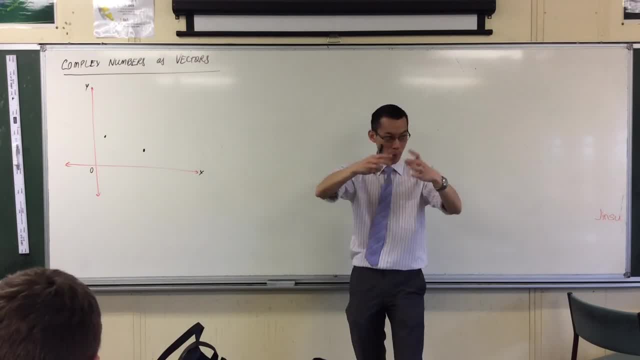 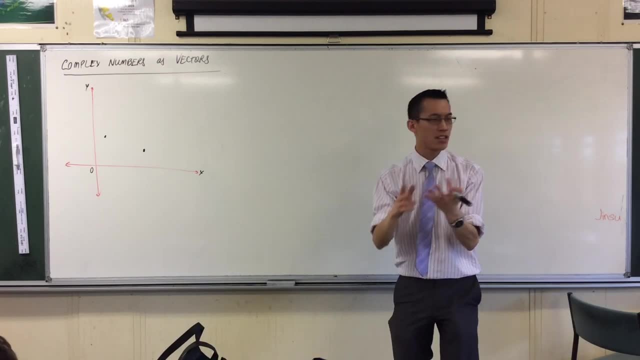 or represent something in a new way, you gain new bonus ideas, right. So, for example, when we went into mod art form, right de Mavres told us there's just this very easy relationship that happens when you raise to a power. 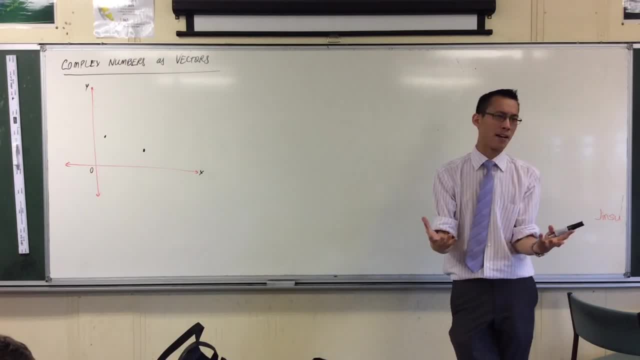 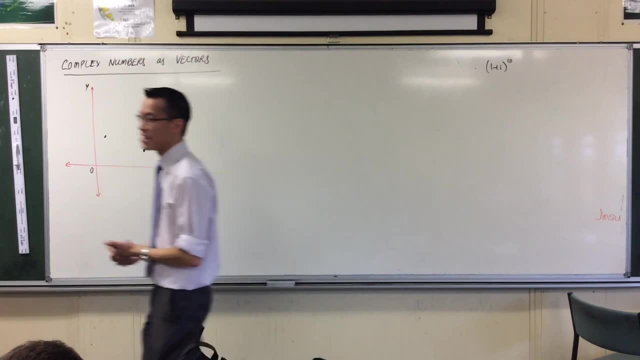 You're just adding angles and going round and round and round, and it's so simple to think about, Whereas if I asked you to do this and all you were equipped with if it was a Cartesian representation, you would be sitting there for a while. 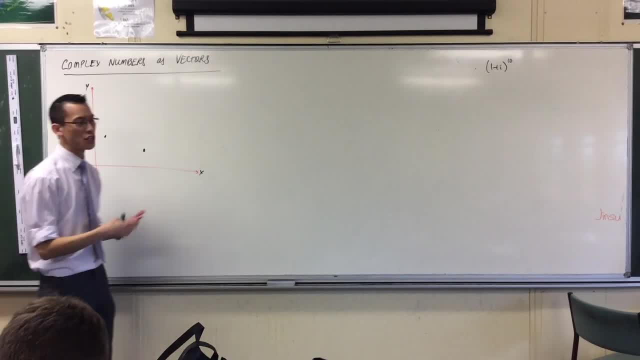 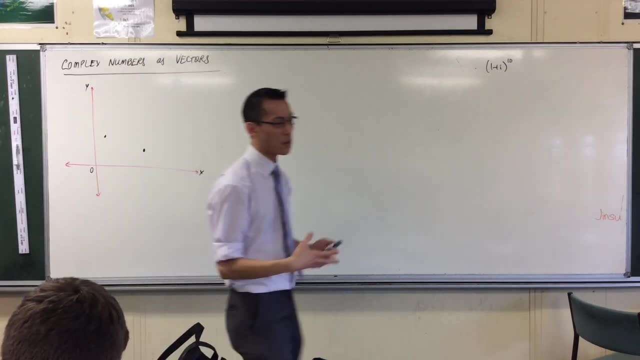 even with binomial theorem. okay, It's just so much more elegant to do it in mod art form. So now we're going to look at yet another way- complex numbers are just so versatile- yet another way of representing them, which again will give us all these extra bonus sort of insights that we'll get. 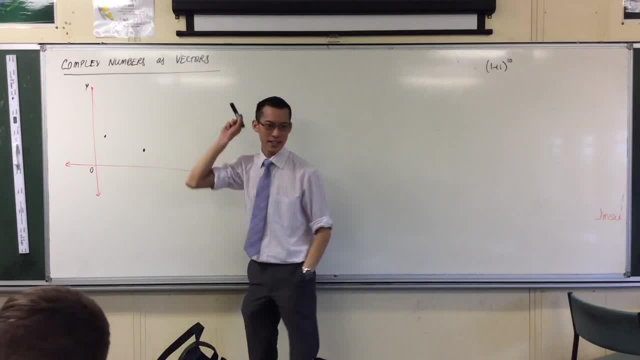 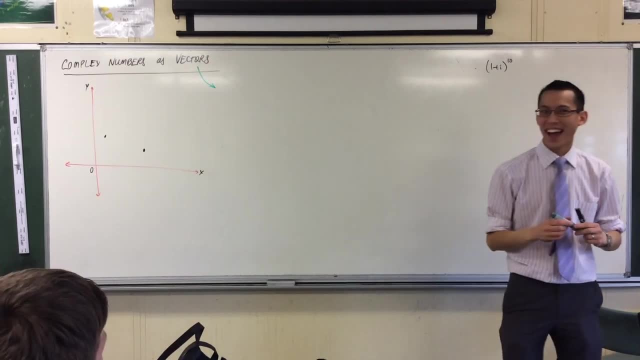 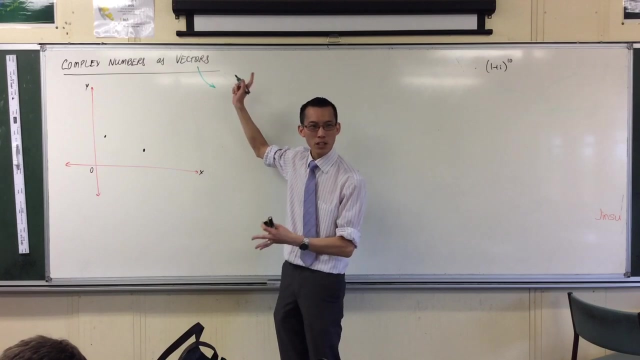 Okay, So complex numbers as vectors. Let's get a definition on the board. What's a vector? A vector is? I was so excited, Me too. Okay, so again two key ideas, right When we were having a look at x plus i, y. 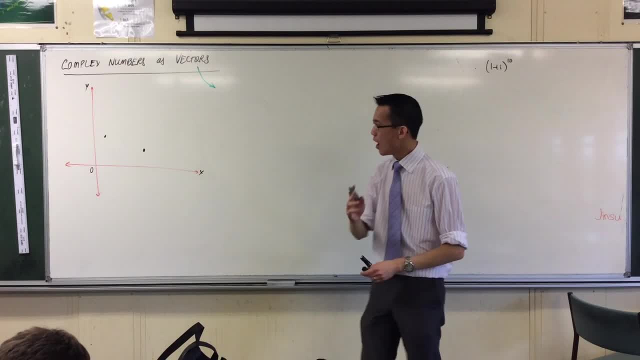 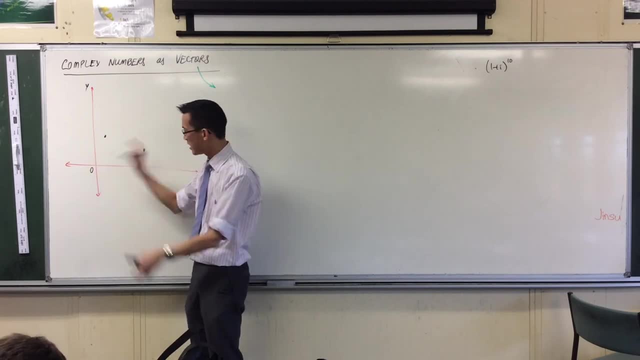 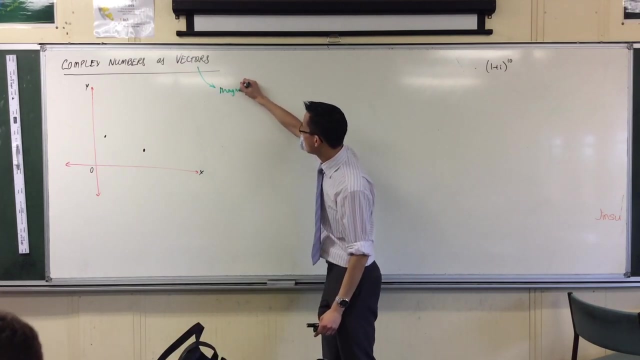 it was just horizontal and vertical, right Horizontal and vertical. When we talked about mod art form, we were talking about modulus, size, distance from the origin and an angle right, This idea that we're about to write down, magnitude and direction. 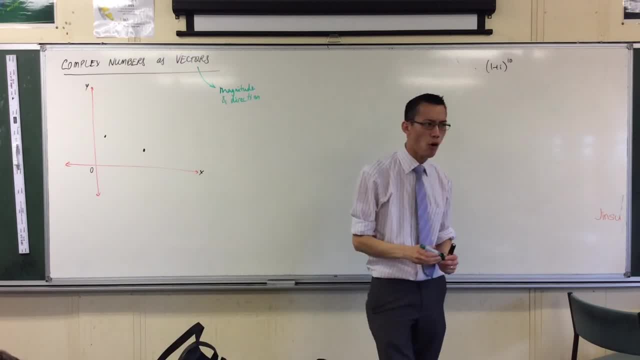 is very, very similar, Like it almost feels like the same thing: Magnitude. what that corresponds to is it's very similar to this idea of modulus right. It's like: how big is this number? Modulus Right? that's what it's related to. 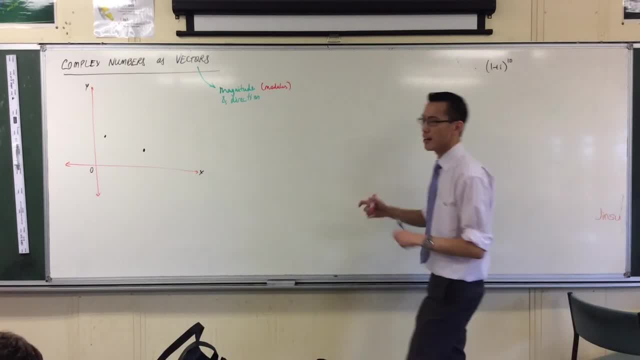 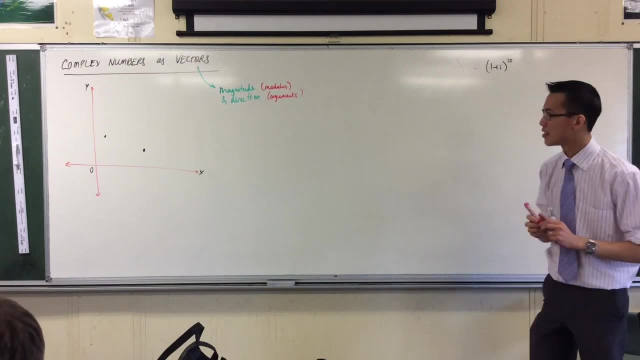 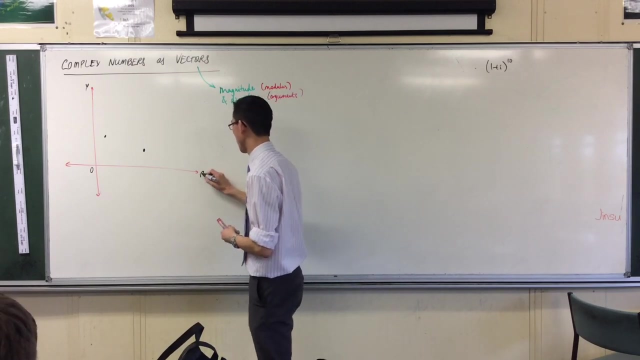 And direction, clearly, is what arguments and angles are about. okay, But there is a subtle difference, and let me try and illustrate it. Yeah, Still the complex one. Oh yeah, Sorry, Old habits die hard. Okay, so we've got real, and 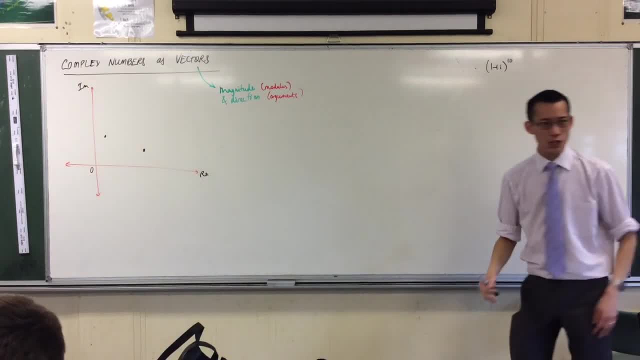 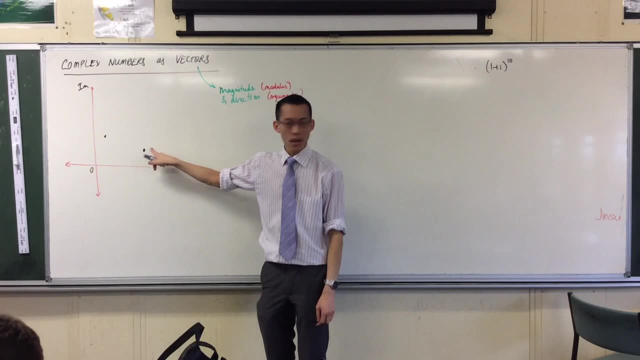 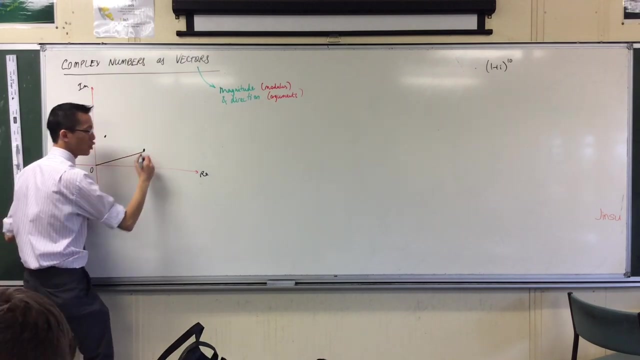 Okay Now, if we think about magnitude and direction, what we're really trying to think about is, rather than complex numbers as a point, like here, it is right- Not so much geometrically the point, but geometrically the interval from one point to another. 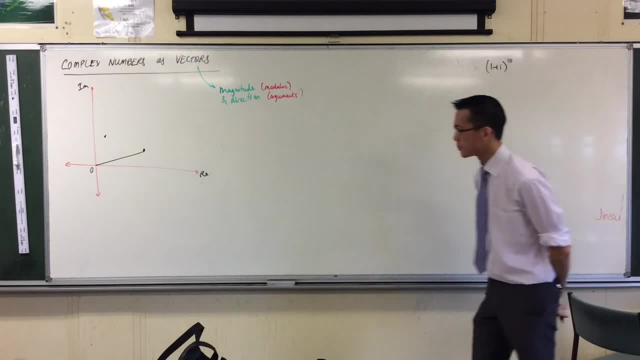 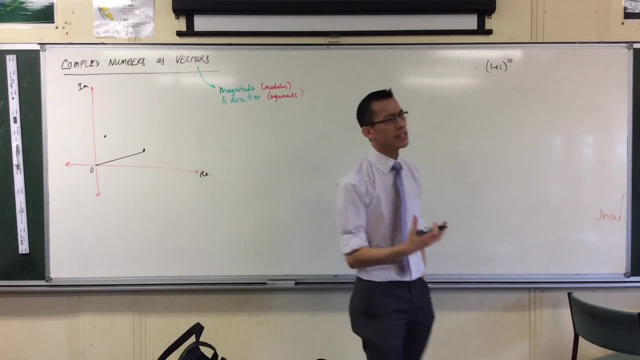 Okay, The interval from one point to another. Okay, Now we would usually call this guy Z1, right, And in fact I will call him Z1 in a second. But if I want an interval, right, I need two points, right. 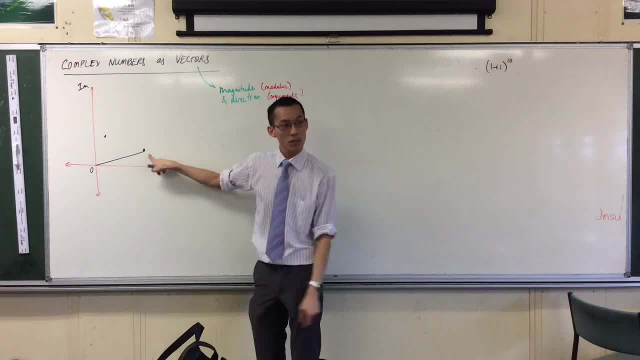 It's like a start and an end, okay. So therefore, I'm not just going to call this Z1, I'm going to give it a name, just like the names we have for all the other points in the past, like a capital letter. 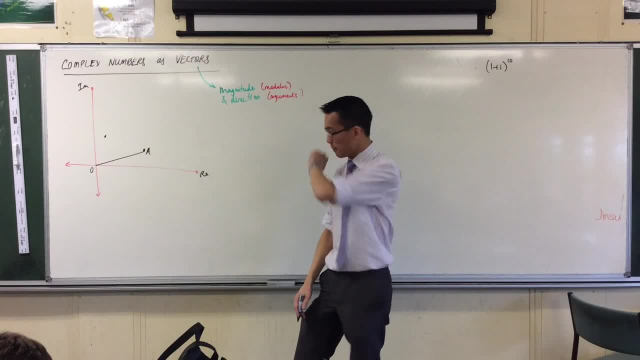 Okay, so I'll call this one, because it's my first one. I'll call it A, but what it represents is my complex number. In this case, I need two of them, so we'll call this one, Z1,, as is our convention. 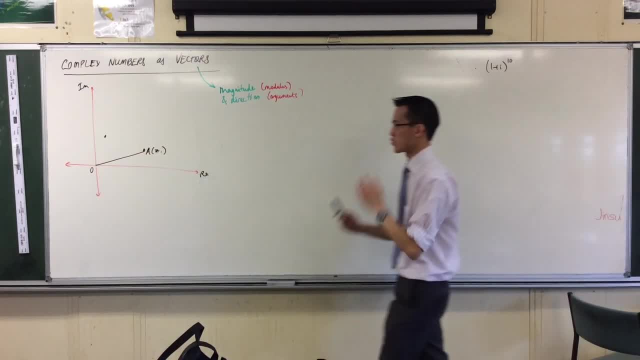 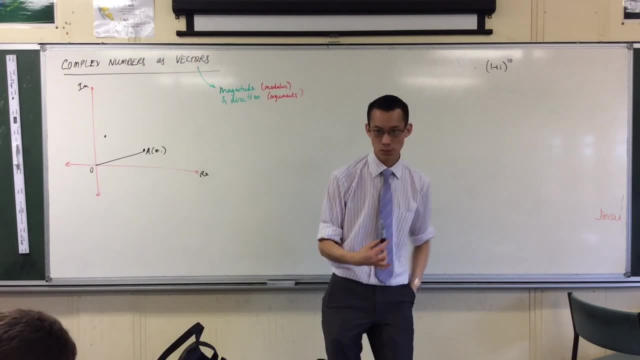 Okay. So now have a look at this right before we talk about this second guy here, In this case here, if I were talking about intervals, intervals, right, I could say OA equals AO, right, Because they're the same interval. 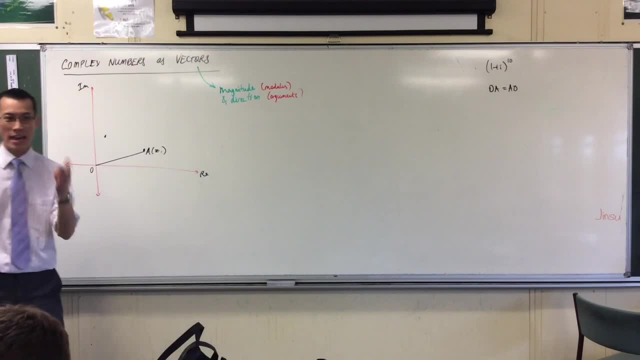 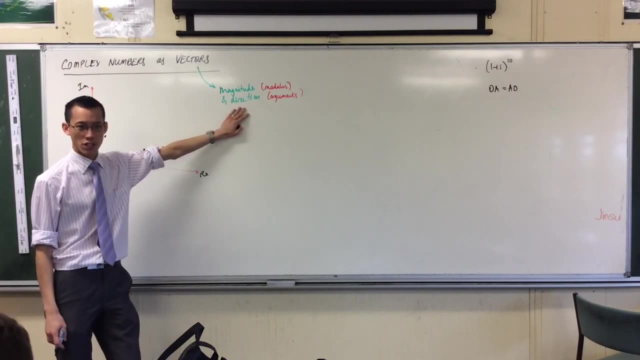 just looked at from two different sides. I start somewhere, I end somewhere, but I end up with the same set of points in between, right, But if you think in terms of direction, direction, and now I'm writing vectors to indicate. 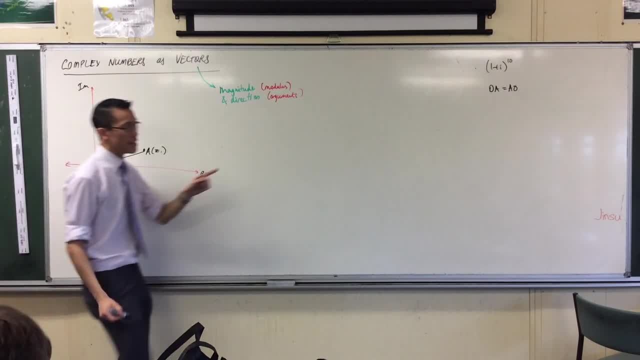 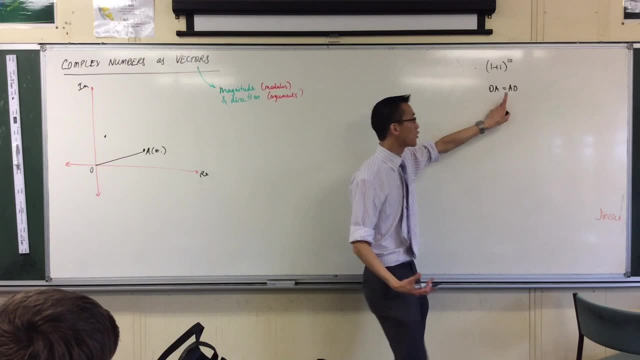 I'm going from one to another right. These things are not the same right. Starting from O and going to A is quite different. In fact, it's literally the opposite of going from A to O. okay, So to indicate that right. 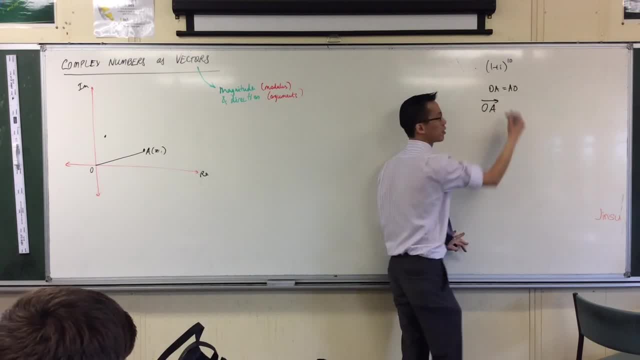 this is with like intervals, but I would say OA and I would put a line with an arrow over the top to indicate vector direction. I'm going somewhere. direction really matters In this case. it's not equal to AO, Okay. 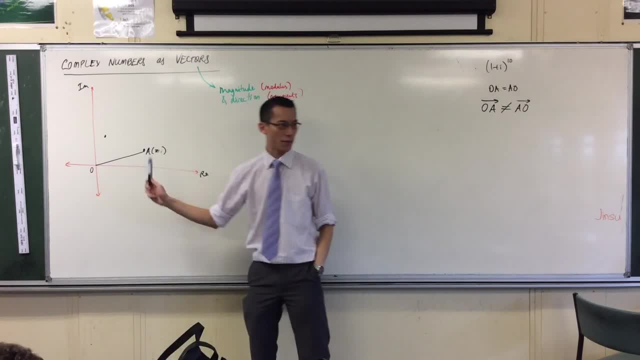 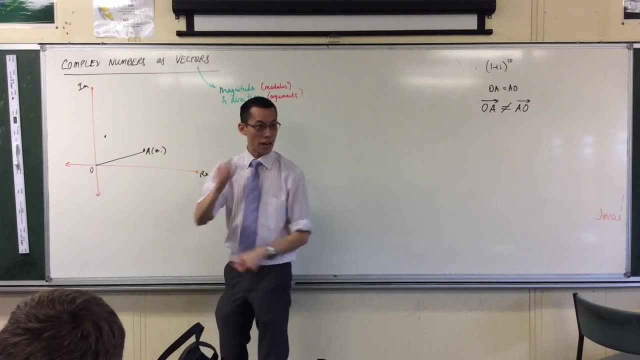 So what have I got here? I've got this vector hanging off here. What's really important, right, is the magnitude, is the length of that. That's fine. The direction is well. I'm going to add an arrow in now. 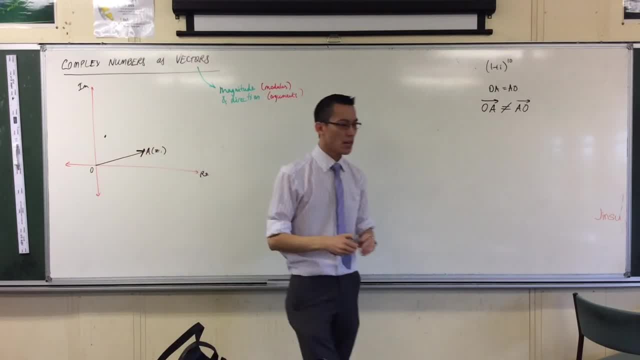 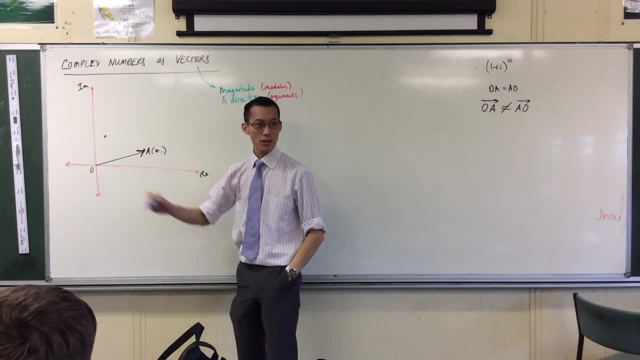 that indicates that way. Don't draw this just yet. We're going to have a few more diagrams to draw on, But if I were to draw, if I were to draw this same interval and an arrow like this right or like this: 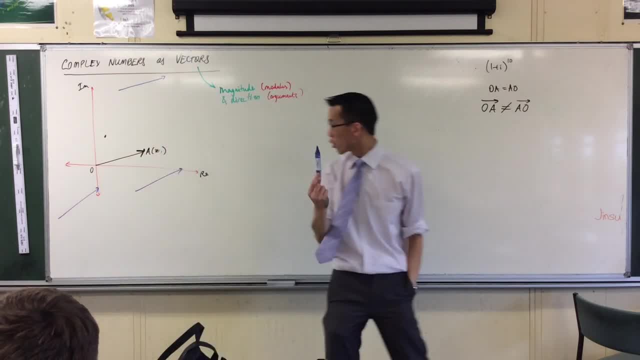 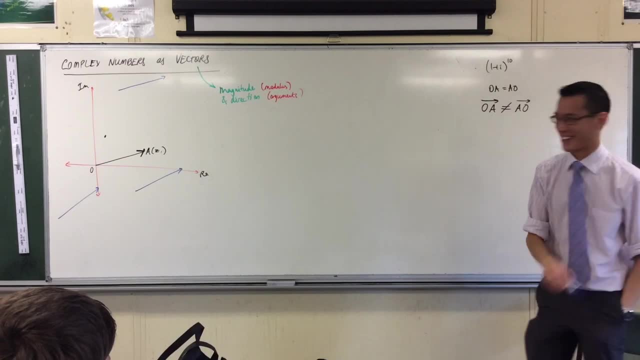 or like this: do you see that all three of these new vectors that I've drawn, you know, within reason? sorry, you know, just keep it better than that. okay, They're all the same magnitude and more or less the same direction. 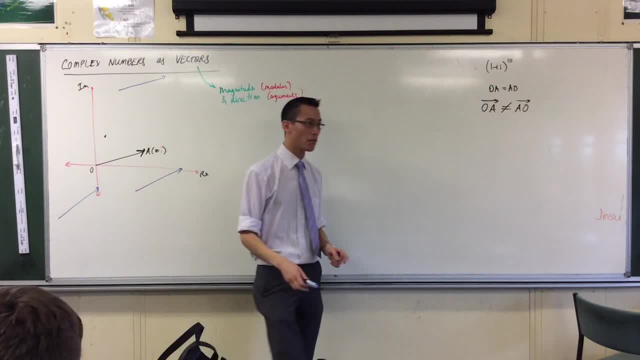 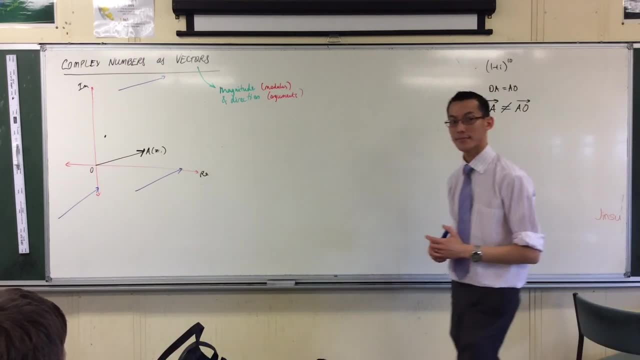 In fact, these vectors are all the same vector. Okay, Yeah, But how can we like, how can we express an imaginary number as, just like, off the off the like, it doesn't have to start from the origin? Yeah, okay. 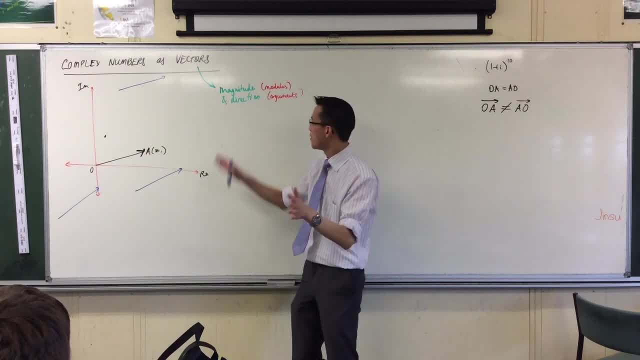 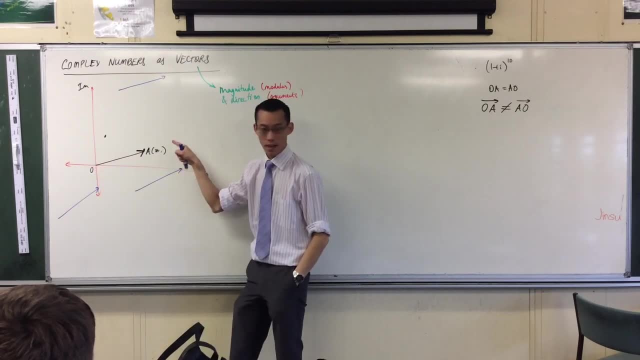 Now here's the whole point. right Point If I'm thinking of back in terms of modulus and argument. right, I am literally, by definition, measuring from here and then you go a distance, and then I measure from here and you go up an angle. 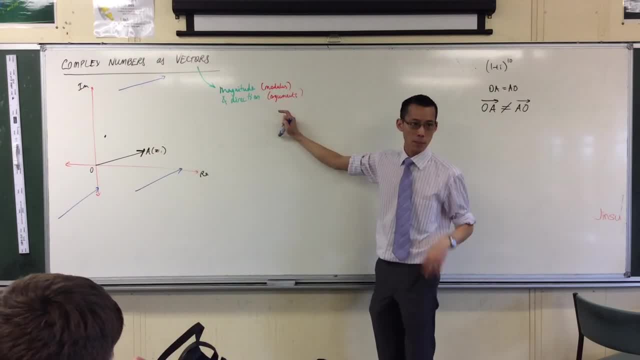 Okay, But a vector is not about modulus and argument, despite how closely related those ideas are. He said that: well, how, how long are you going to, how far are you going to take me away, And which way do you want to take me? 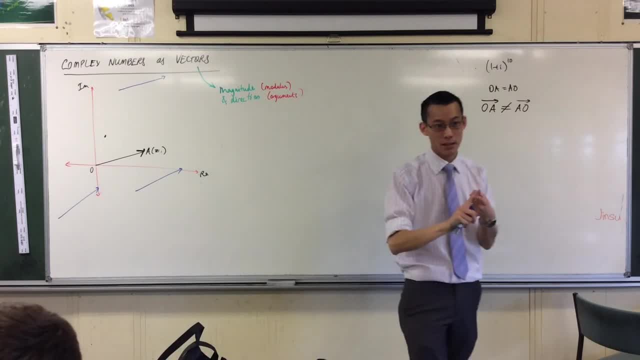 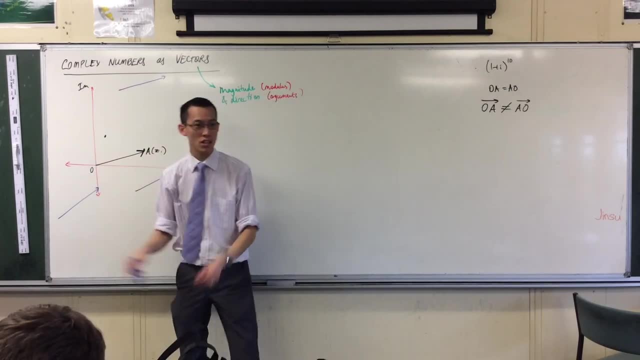 Right, And they don't care about where you begin. or well, yeah, because they don't care about where you begin. there's not a positive real axis that you're measuring from and there's no origin that you begin from. They're all the same vector. 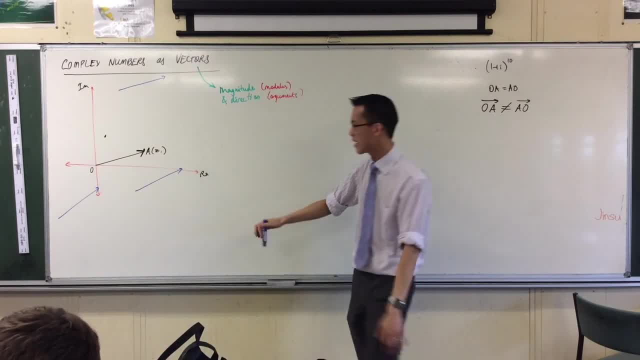 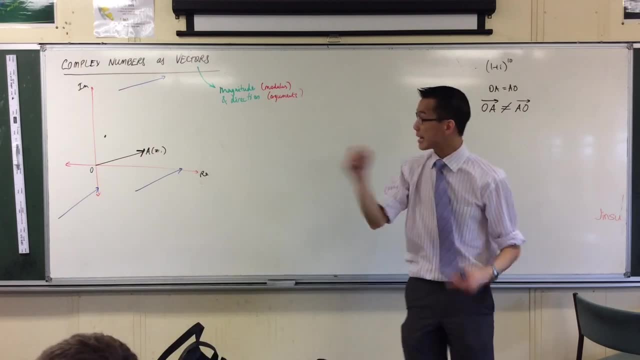 Now we do distinguish between them, and I'll introduce some language to show you that. But just this idea of focusing on the actual interval as opposed to focusing on the point, that's the key difference between thinking of that as vectors or as points on a plane. 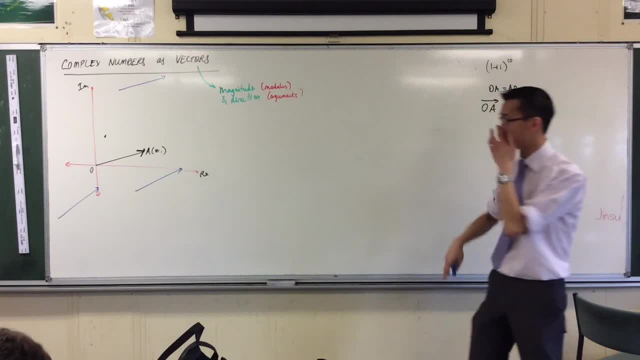 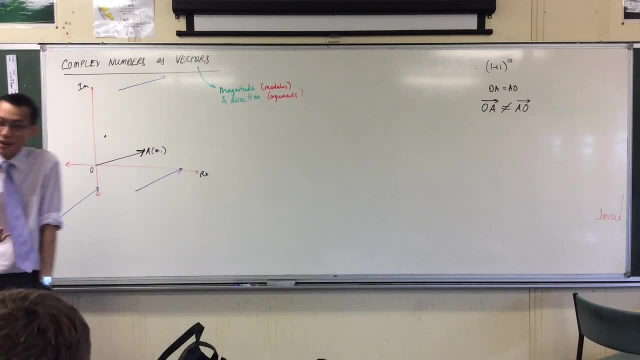 Okay, All right. So magnitude and direction. There's A Z1.. Let's put. let's put Z2 on here and again. because I want to have some language that borrows my language of points, I'm going to call it B. 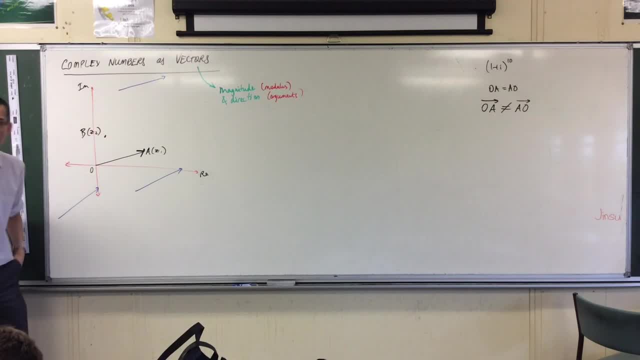 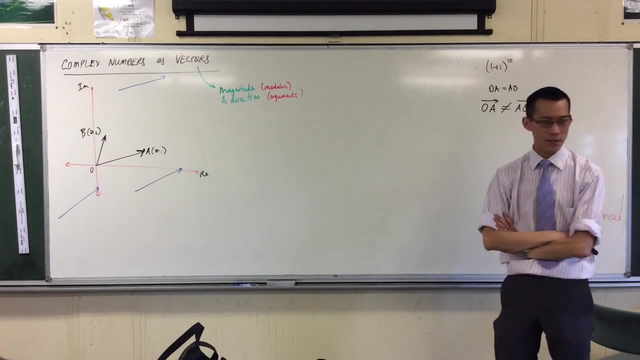 Very unoriginal. Okay Now, if B is up here, then OB would be this vector. Okay, Now, borrowing what you already know about complex numbers and how you add them and what that means geometrically, Okay, For instance, just as a first example. 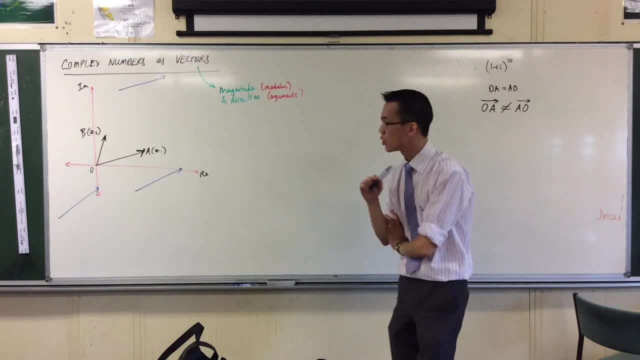 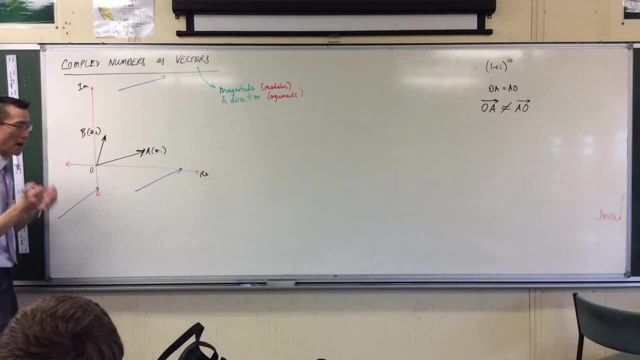 where would Z1 plus Z2? where would it be on this diagram? Okay, Now with our parallelogram law, I have a parallelogram. In fact, I'm even going to draw a parallelogram on here. What I'm going to do is: 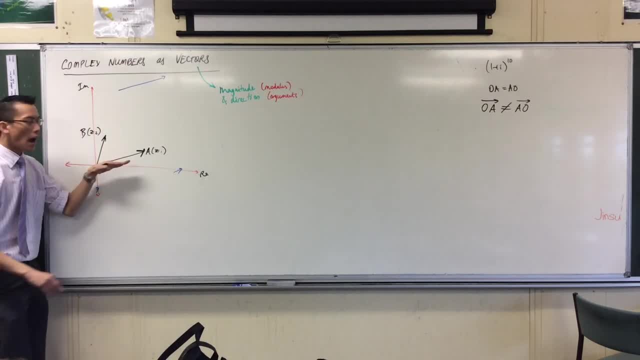 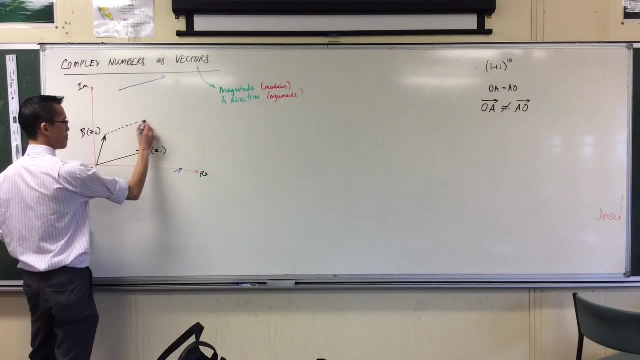 now that I have this vector language- let me get these guys out of here- I can take this OA vector OA And if I move it up here, like so, reposition it, then adding these two complex numbers together is the same as stringing two vectors together. 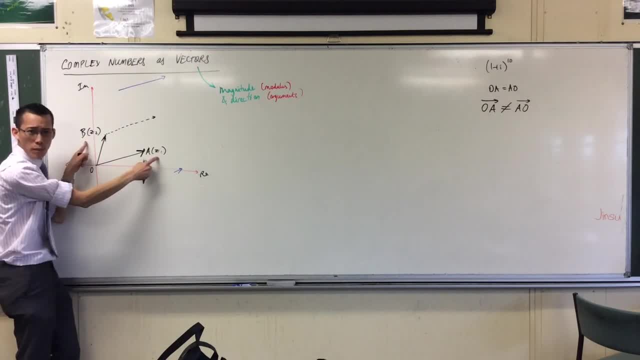 Can I say that again, That's important. Adding these two complex numbers together is the same as doing one vector and stringing it together with another one. Right, It's like step one, step two, Or because addition is still commutative. 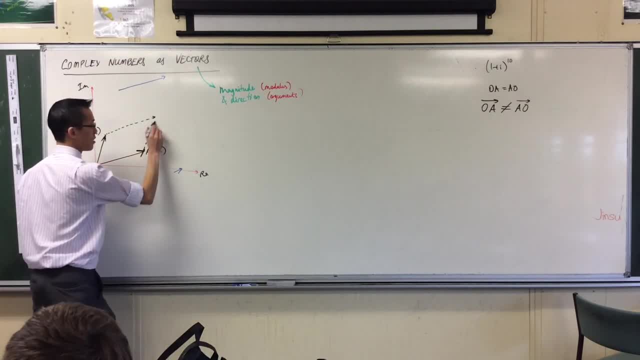 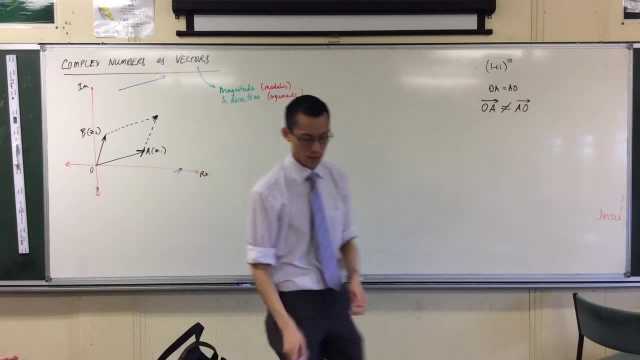 right, I can do step two and then step one. I'm still going to get there. Okay, So I've got this new point up here, which means I have a new vector. Okay, So, color Where's blue? 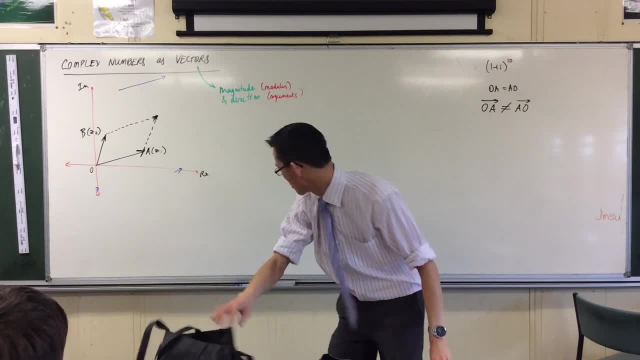 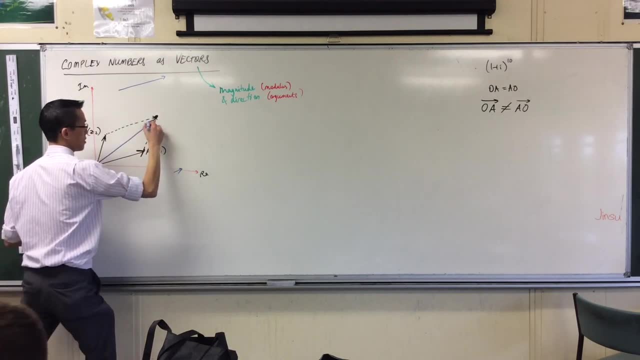 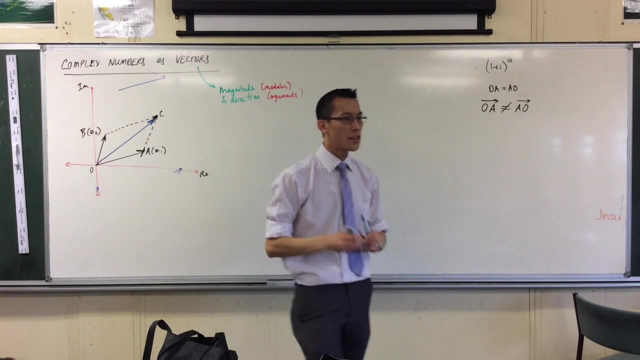 It has blue. It has blue, It's there. Oh, okay, Of course, There you go, All right, So Okay. So what I've got in blue there, if we call this point C, the vector OC. 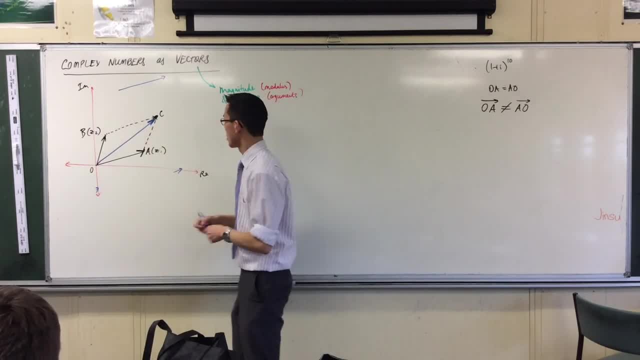 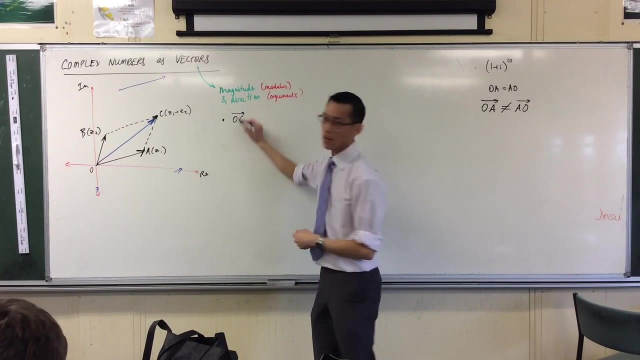 that represents the vector Z1 plus Z2.. All right, No, I'll stay with that. So let's formalize some of this. I'm going to give you some new language for it. I'm going to say OC and I'm going to put that line over the top. 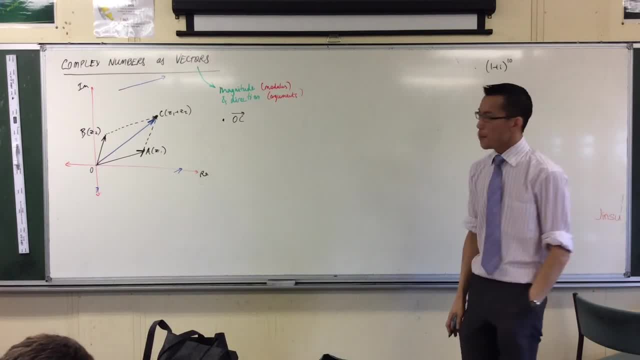 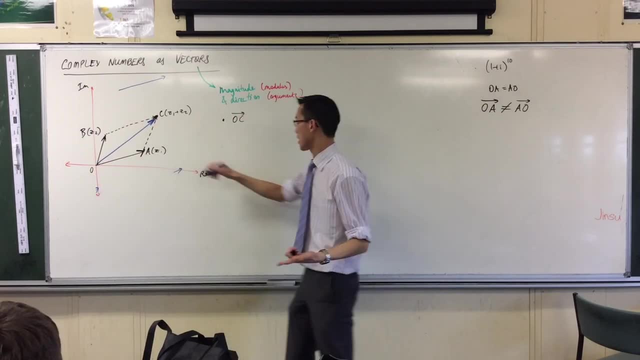 to indicate it's a vector. It's got a direction Right, Because OC is from the origin. okay, it's from the origin. it gives me the position over here, So it's called the position vector. All right, It's the position vector. 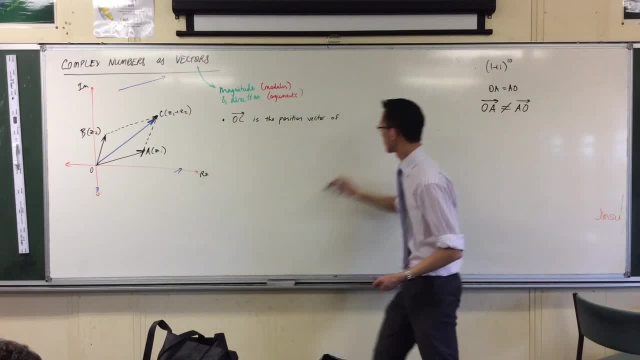 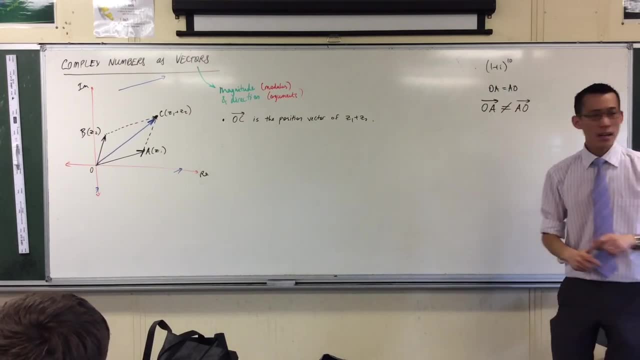 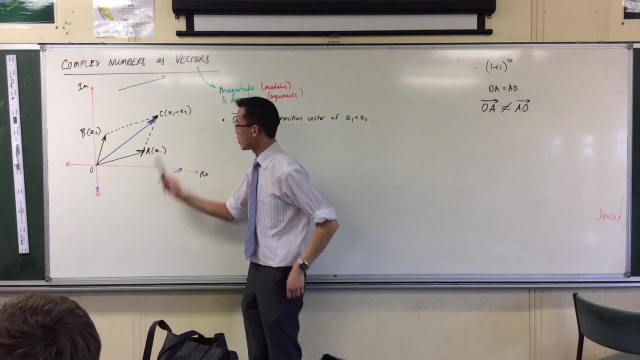 of Z1 plus Z2.. All right, Excuse me. In addition to that, remember we said: oh, you know, you've got this parallelogram happening here, Right, OACB. So immediately like: what is this blue shape? 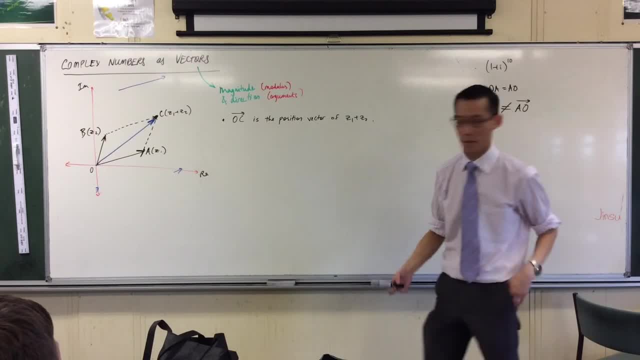 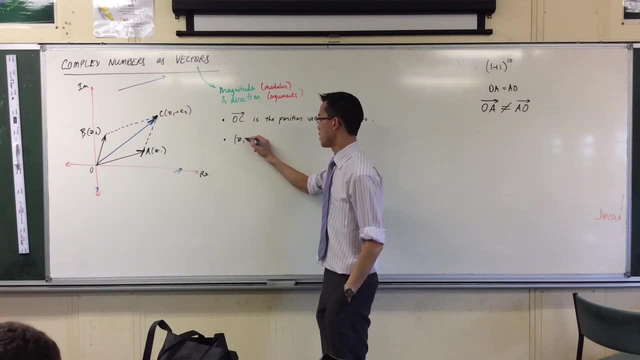 It's a diagonal of this parallelogram. Right, So I can say the magnitude of this vector here. Right, And that vector represents Z1 plus Z2.. Right, So I can still use my same modules notation because it's referring to the same numbers.